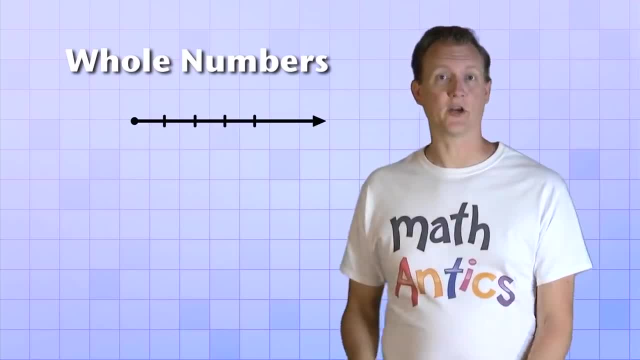 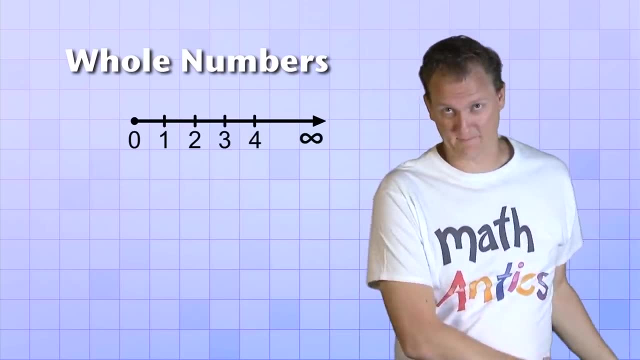 what whole numbers are right? They're the set of numbers on the number line, starting with zero and then counting up one at a time: one, two, three, four, all the way to infinity. That's a lot of numbers, but it's only half the story, And that's because the number 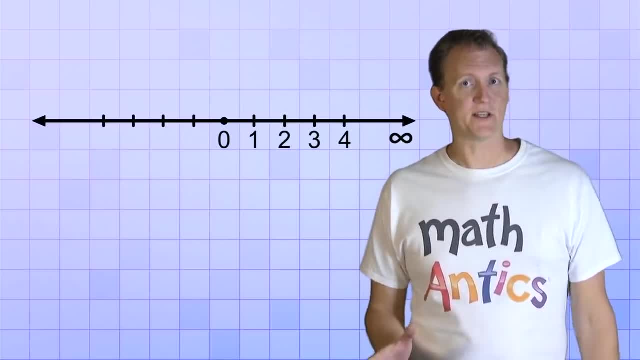 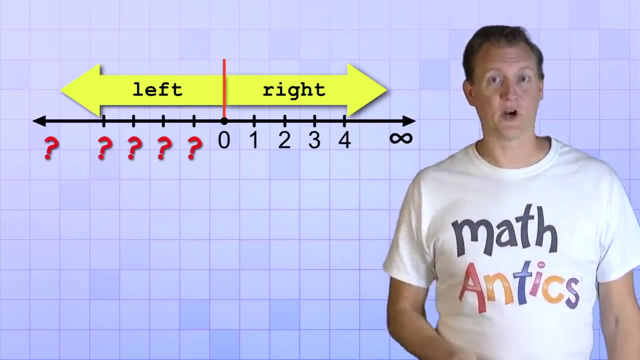 line really goes in both directions. You're used to seeing the number line starting at zero and just going to the right, but the number line also goes to the left. And what numbers are on that part of the number line? Yep, you guessed it… negative numbers. 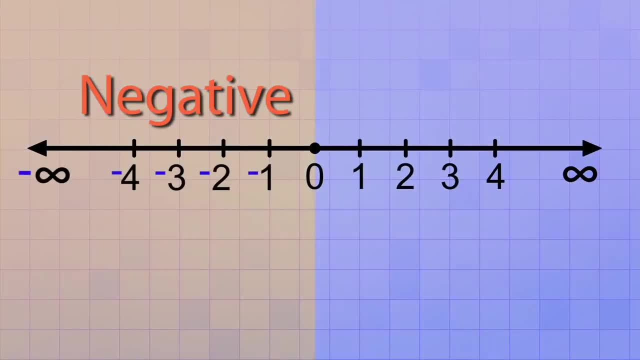 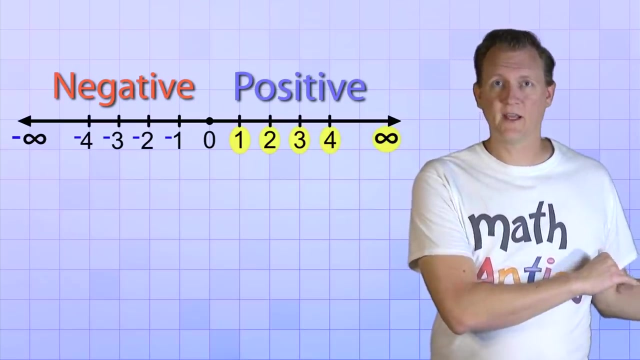 The negative numbers are just like numbers. They're like a mirror image of the numbers on the right side of the number line that we call the positive numbers, And zero is the special number that separates the positive numbers from the negative numbers. By the way, when you combine all these numbers- one, two, three and so on, up to infinity- 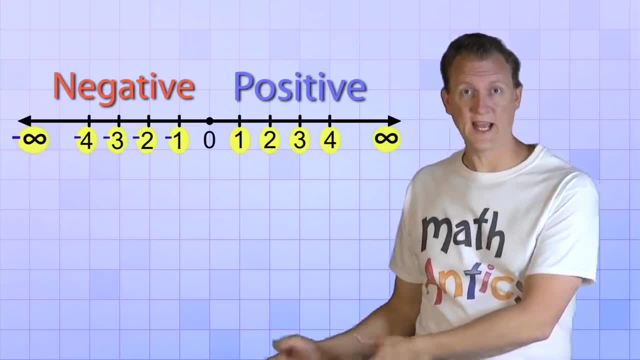 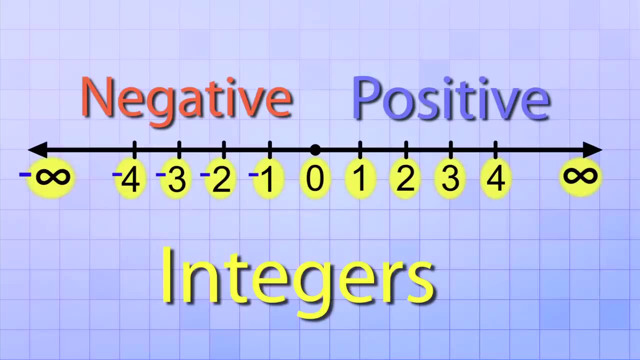 and negative one, negative two negative three and so on, down to negative infinity and the number zero. that entire set of numbers gets a special name in math: They're called the integers. As you can see, the negative numbers look just like the numbers on the right side of. 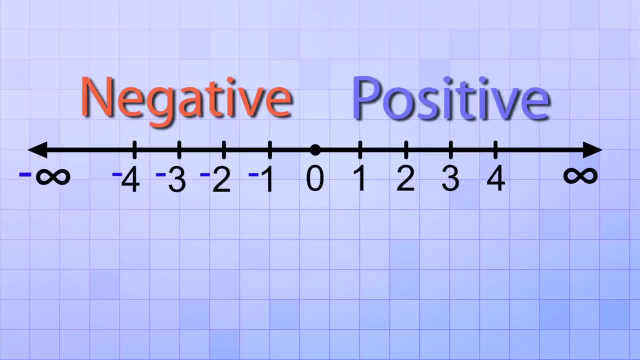 the number line. The only difference is that they have a negative sign in front of them. The negative sign looks just like the minus sign. In fact, if we wanted to, we could write a positive sign, a plus, in front of all the positive numbers, But to save time we just 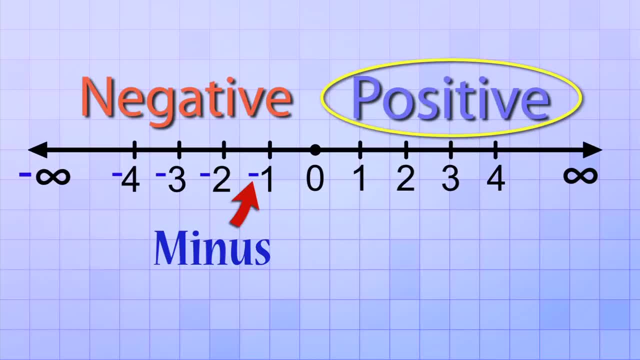 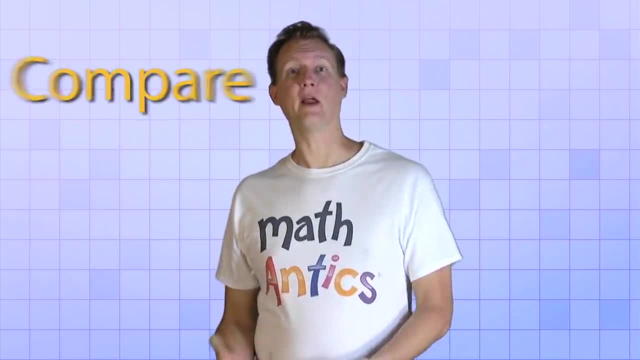 assume that if a number doesn't have any sign in front of it, then it's positive. Positive is the default sign. Okay, now that you know what negative numbers are, we need to learn how to compare them to other integers. Remember that in math you can't just write a positive sign in front. 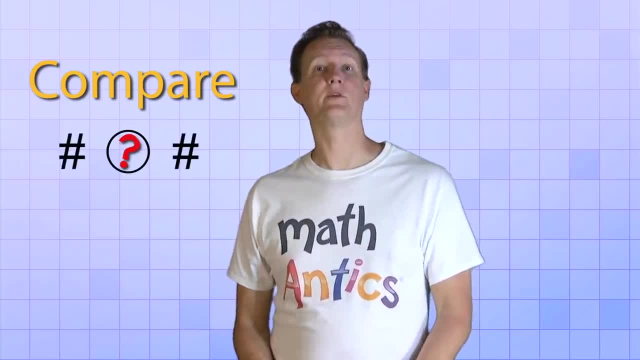 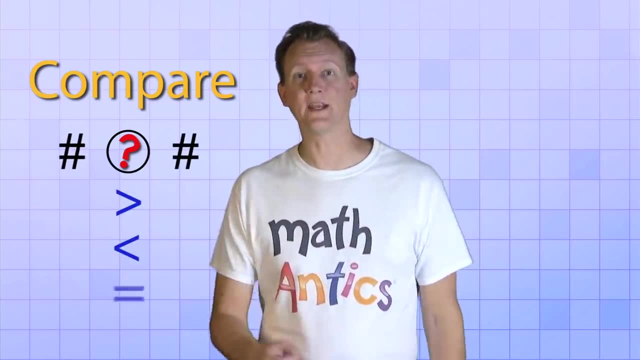 of a positive number, You need to learn how to compare them to other integers. Remember that in math, comparing just means saying which of two numbers is bigger or smaller than the other, or saying that they're equal, And to do that we use the greater than, less than or equal. 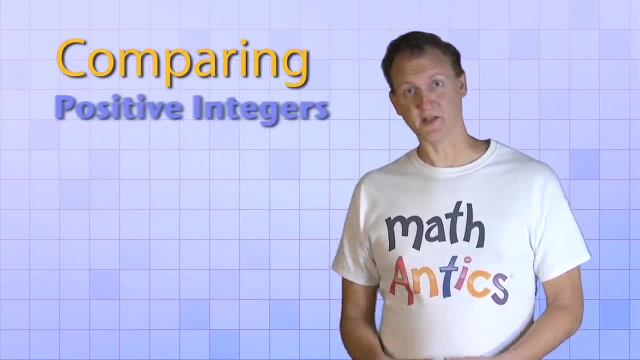 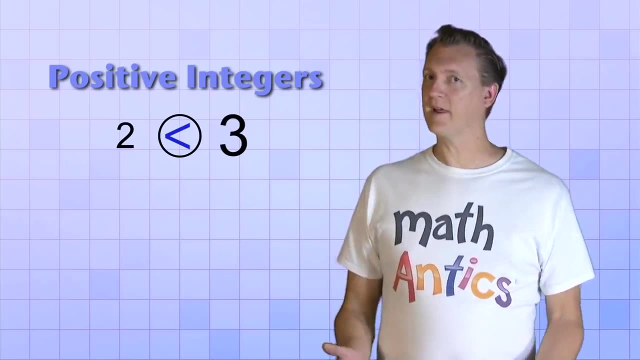 signs. You're probably already pretty good at comparing positive integers, Like if I ask which is bigger- 2 or 3? You know that 3 is bigger than 2.. But what if I ask you to compare two negative integers? Which is bigger- Negative 2 or negative 3?? 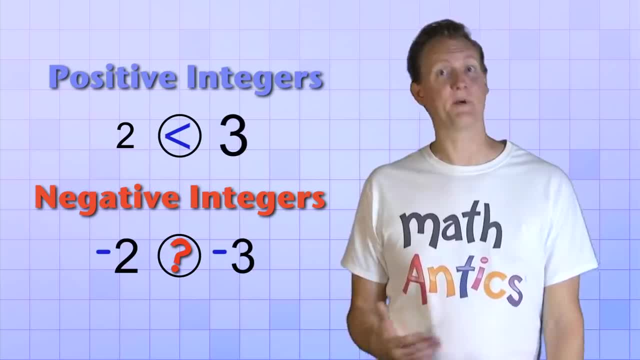 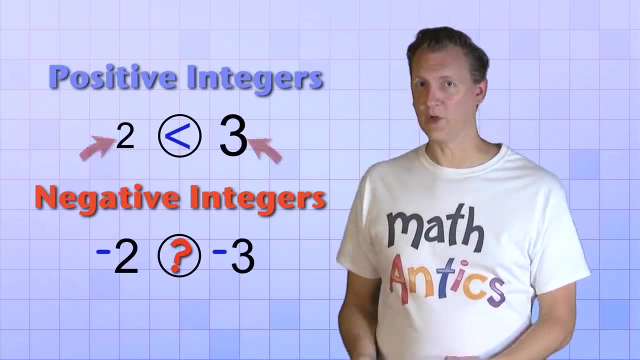 Ah, this is where negative numbers can be a little tricky, Especially if this is your first time learning about them. That's because you're so used to 3 being bigger than 2, that when you see negative 2 and negative 3,. 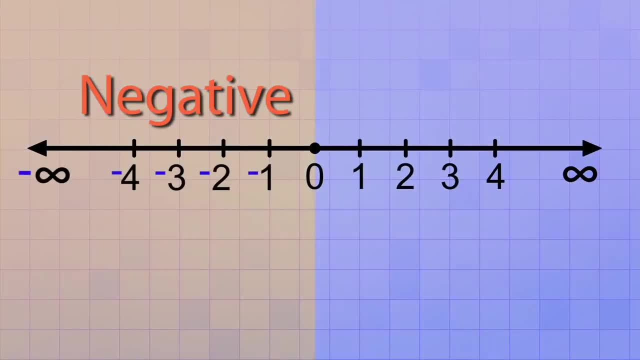 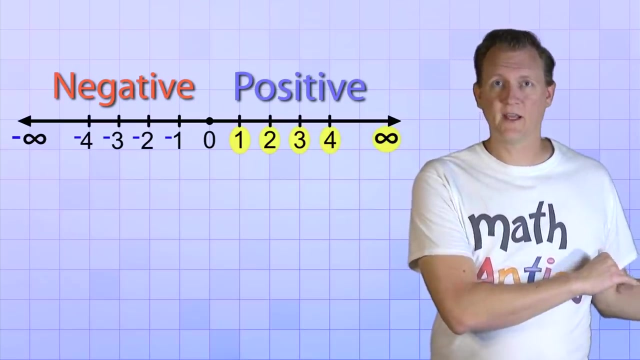 The negative numbers are just like numbers. They're like a mirror image of the numbers on the right side of the number line that we call the positive numbers, And zero is the special number that separates the positive numbers from the negative numbers. By the way, when you combine all these numbers- one, two, three and so on, up to infinity- 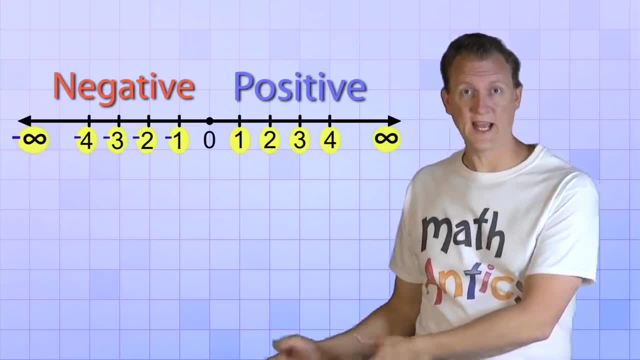 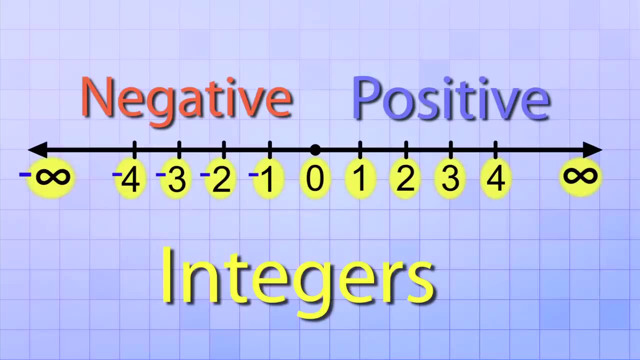 and negative one, negative two negative three and so on, down to negative infinity and the number zero. that entire set of numbers gets a special name in math: They're called the integers. As you can see, the negative numbers look just like the numbers on the right side of. 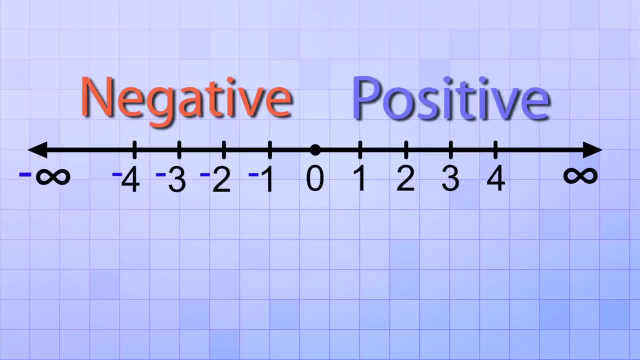 the number line. The only difference is that they have a negative sign in front of them. The negative sign looks just like the minus sign. In fact, if we wanted to, we could write a positive sign in front of all the positive numbers, But to save time we just 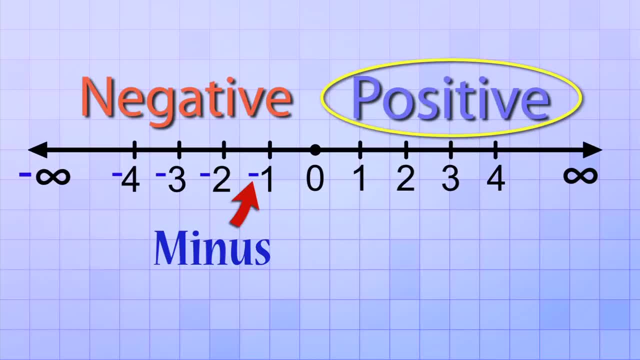 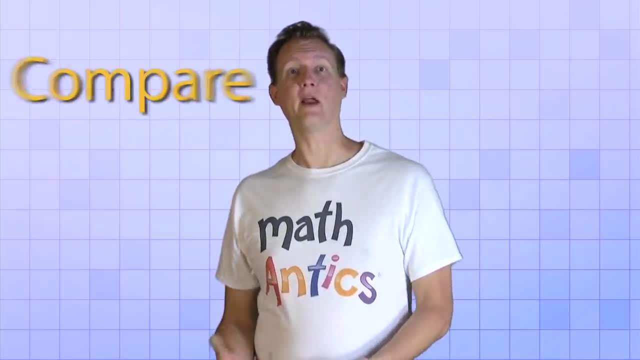 assume that if a number doesn't have any sign in front of it, then it's positive. Positive is the default sign. Okay, now that you know what negative numbers are, we need to learn how to compare them to other integers. Remember that in math, you need to know how to compare them to other. 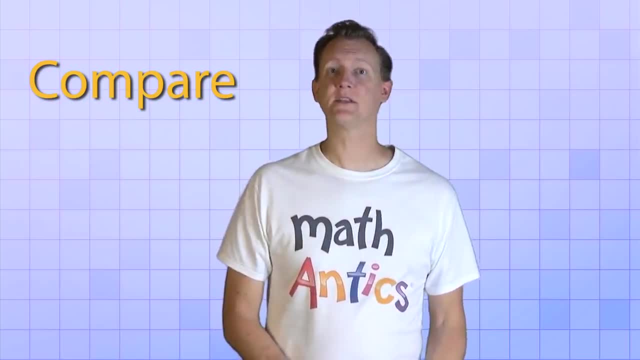 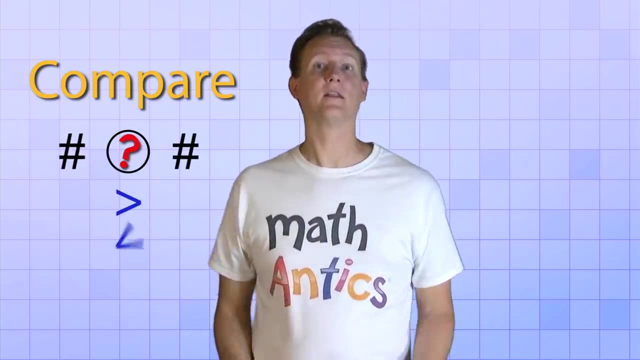 integers. Okay, now that you know what negative numbers are, we need to learn how to compare them to other integers. Remember that, in math, comparing just means saying which of two numbers is bigger or smaller than the other, or saying that they're equal, And to do that we use the greater than less. 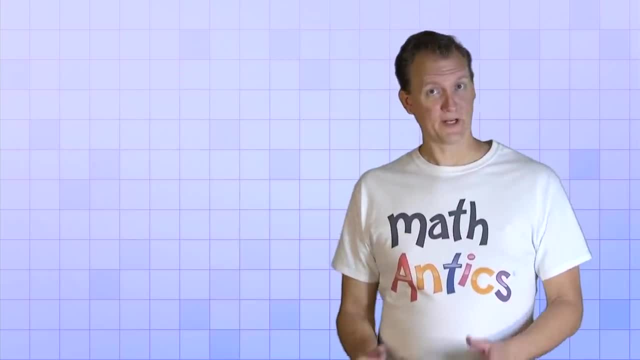 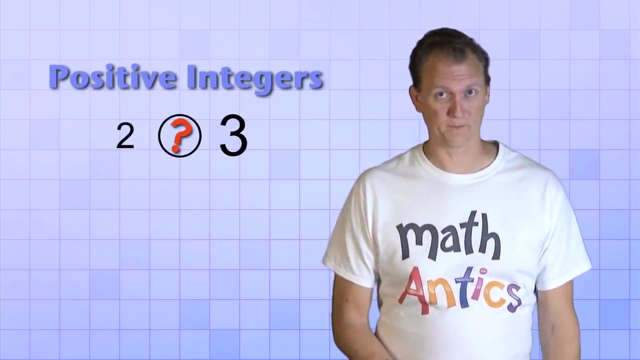 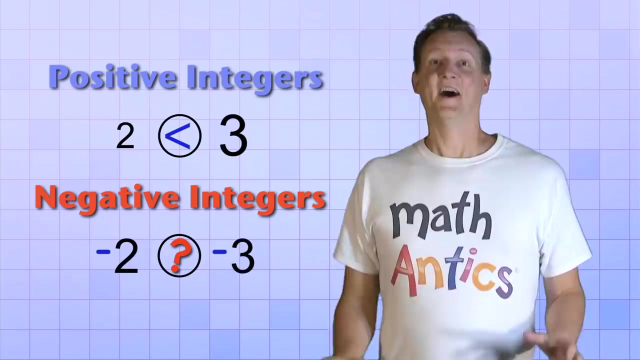 than or equal signs. You're probably already pretty good at comparing positive integers. Like if I ask which is bigger, Two or three, You know that three is bigger than two. But what if I ask you to compare two negative integers? Which is bigger- Negative two or negative three? 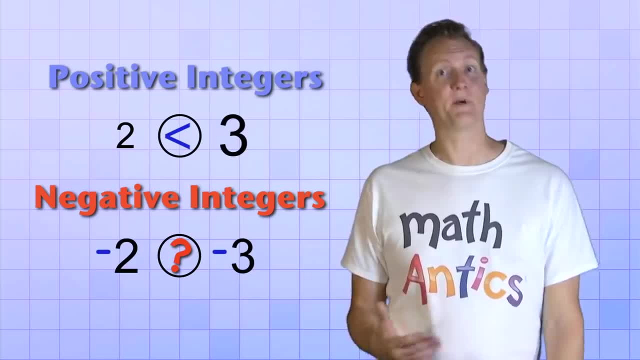 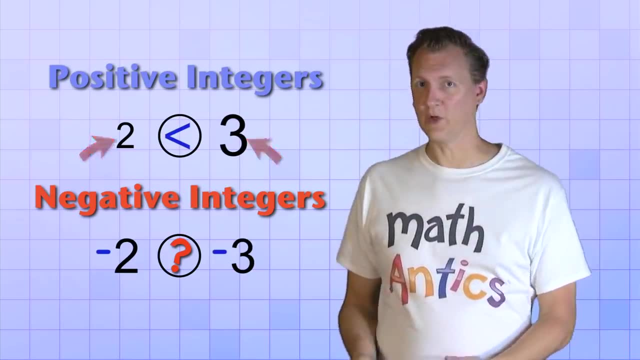 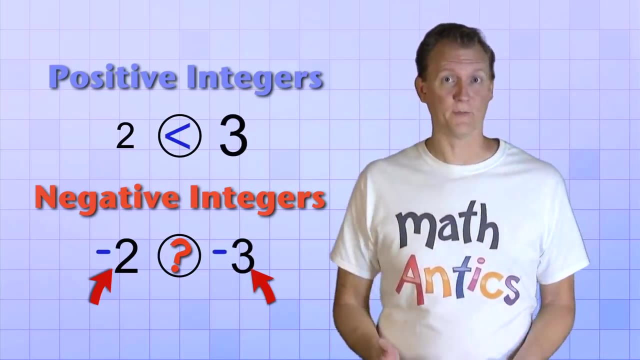 Ah, this is where negative numbers can be a little tricky, Especially if this is your first time learning about them. That's because you're so used to three being bigger than two that when you see negative two and negative three, it's really tempting to think that negative three must be bigger than negative two. But it's not. 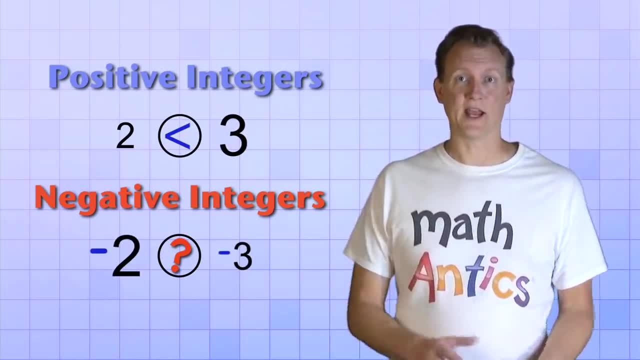 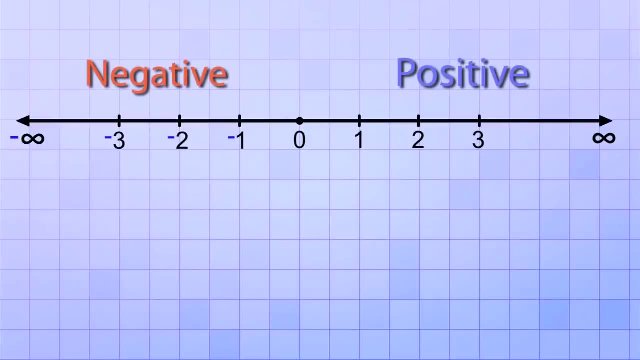 Negative three is actually smaller or less than negative two. And to help you understand why, let's look at our number line again. Have you noticed that if you start at zero on the number line, then you move to the right. the numbers keep getting bigger and bigger as you go along? 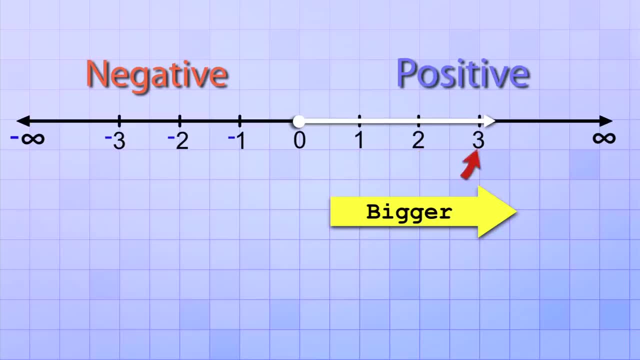 1 is greater than 0,, 2 is greater than 1, and 3 is greater than 2, and so on. But what if we go in the opposite direction, instead to the left? As we go to the left, the numbers get smaller and smaller. 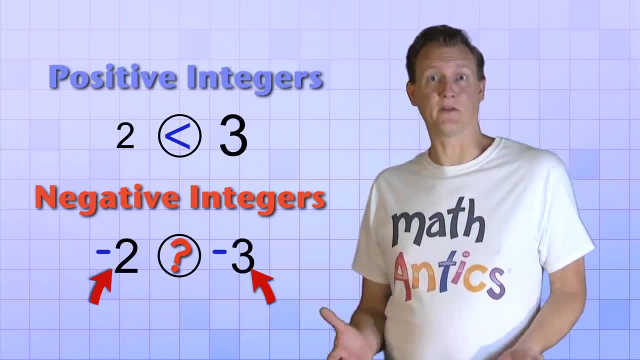 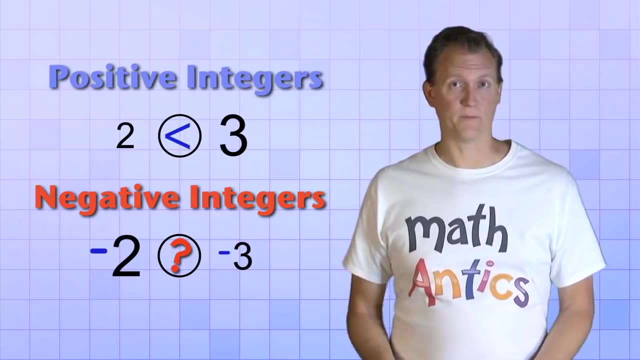 it's really tempting to think that negative 3 must be bigger than negative 2.. But it's not. Negative 3 is actually smaller or less than negative 2.. And to help you understand why, let's look at our number line again. 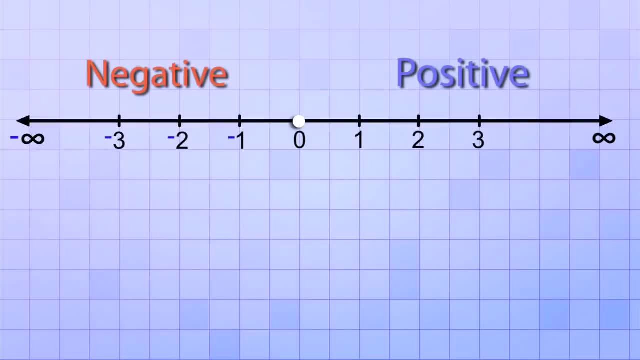 Have you noticed that if you start at zero on the number line and then you move to the right, keep getting bigger and bigger as you go along? 1 is greater than 0,, 2 is greater than 1, and 3 is greater than 2, and so on? 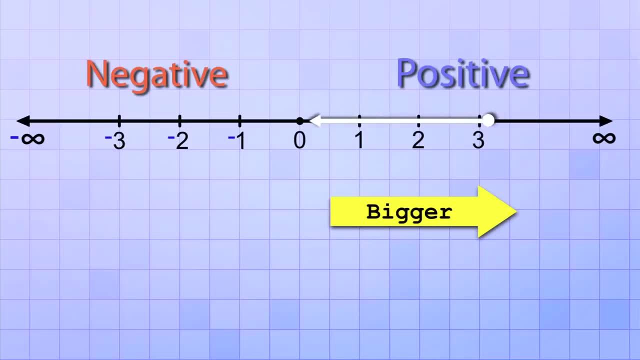 But what if we go in the opposite direction, instead to the left? As we go to the left, the numbers get smaller and smaller: 2 is less than 3,, 1 is less than 2, and 0 is less than 1.. 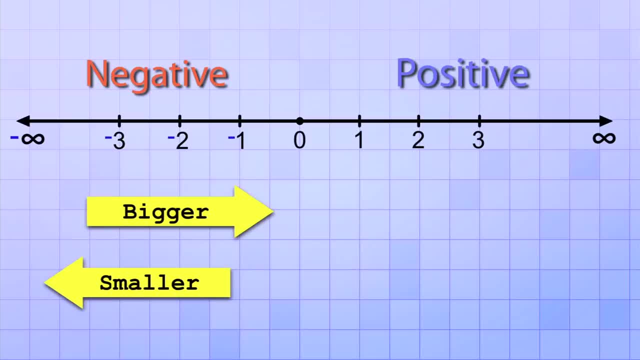 Well, those same exact rules apply to the negative side of the number line also. The numbers get bigger as you go to the right and they get smaller as you go to the left. So since negative 3 is on the left side of negative 2, it's actually smaller than negative 2.. 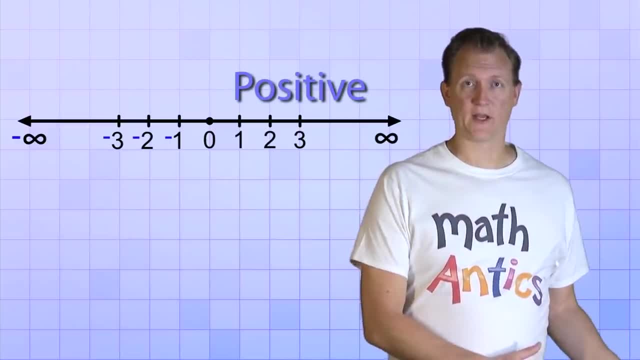 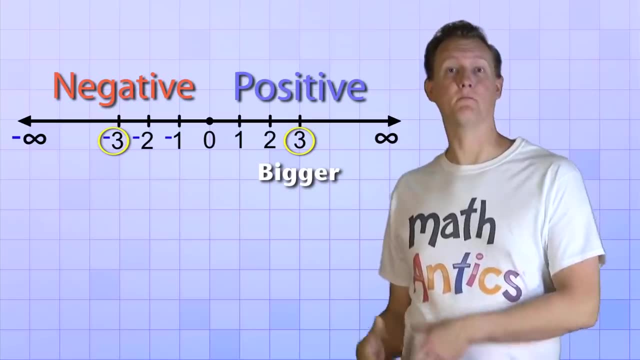 I like to think of it like this: On the positive side of the number, line, 3 is more positive than 2, so it's bigger. But on the negative side of the number, line negative 3 is more negative than negative 2, so it's smaller. 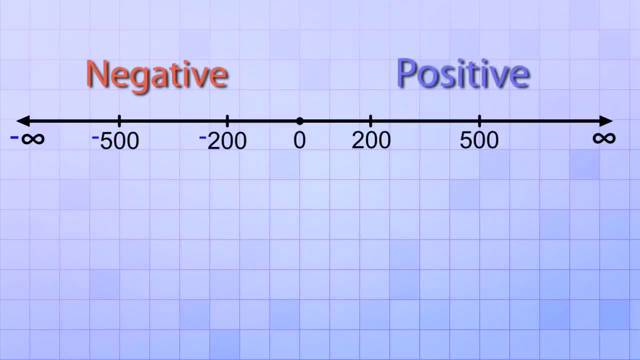 And you can use that idea, no matter what the numbers are. On the positive side, 500 is more positive than 200, so it's bigger, But on the negative side, negative 500 is more negative than negative 200, so it's smaller. 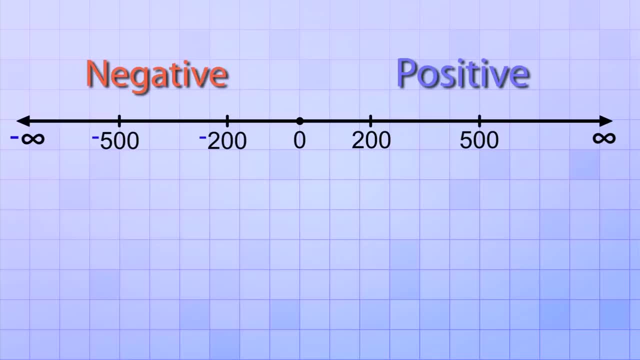 Keep that in mind if anyone ever offers to give you negative $500.. The 500 part sounds pretty good, but the negative part… not so much. Alright, so the positive integers are on the right side of 0 on the number line. 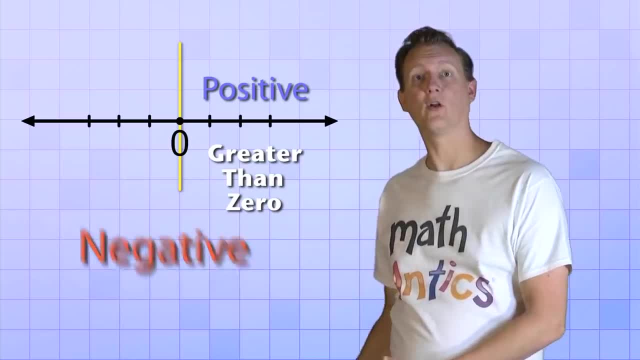 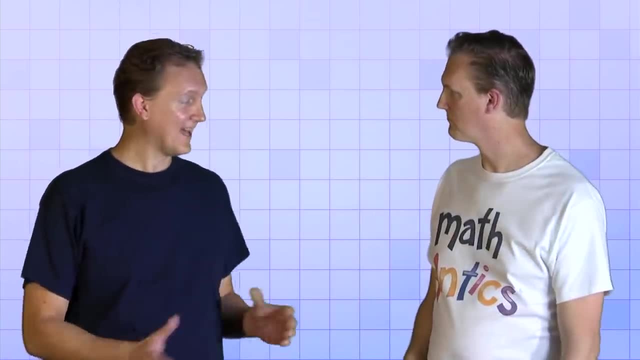 which means they're all greater than 0. And the negative integers are all on the left side of 0 on the number line, which means they're all less than 0. What Hold on a second Less than 0?? How can any number be less than 0?? 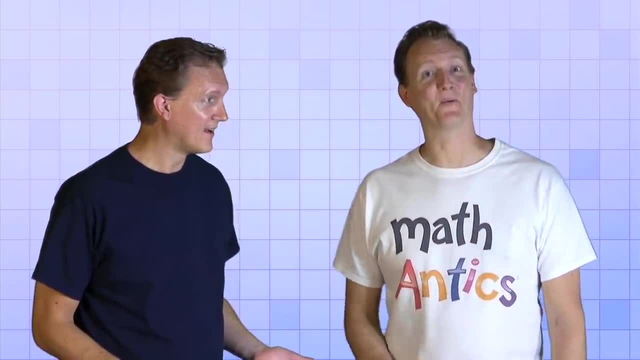 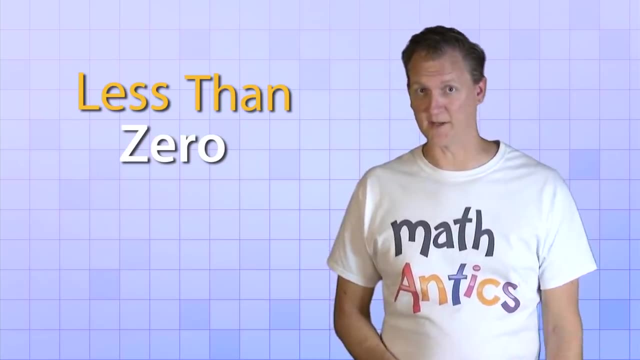 I mean, doesn't 0 mean nothing? Ugh, that's a good question. At first it can be hard to see how there could be numbers that are less than 0. But here's an example that will help you understand. 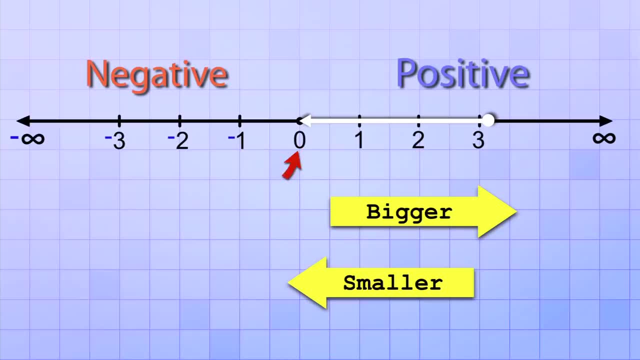 2 is less than 3,, 1 is less than 2, and 0 is less than 1.. Well, those same exact rules apply to the negative side of the number line also. The numbers get bigger as you go to the right and they get smaller as you go to the left. 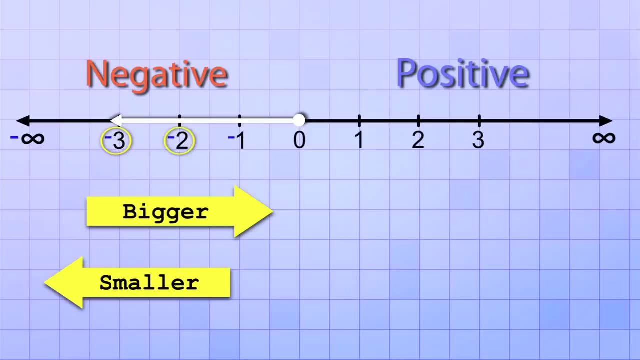 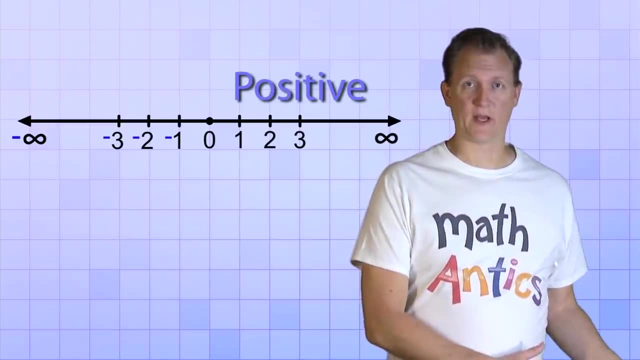 So since negative 3 is on the left side of negative 2, it's actually smaller than negative 2.. I like to think of it like this: On the positive side of the number, line 3 is more positive than 2, so it's bigger. 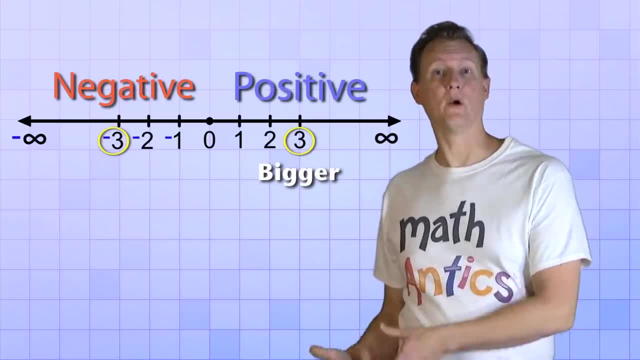 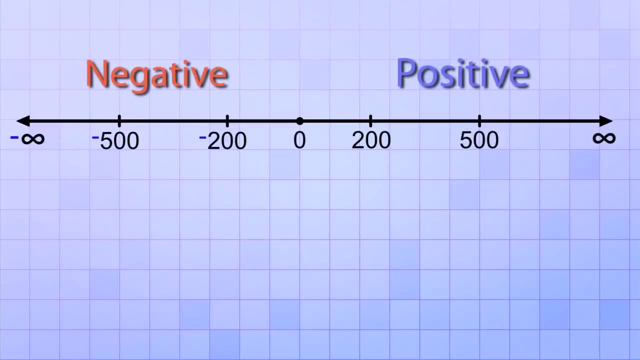 But on the negative side of the number line, negative 3 is more negative than negative 2, so it's smaller, And you can use that idea, no matter what the numbers are. On the positive side, 500 is more positive than 200, so it's bigger. 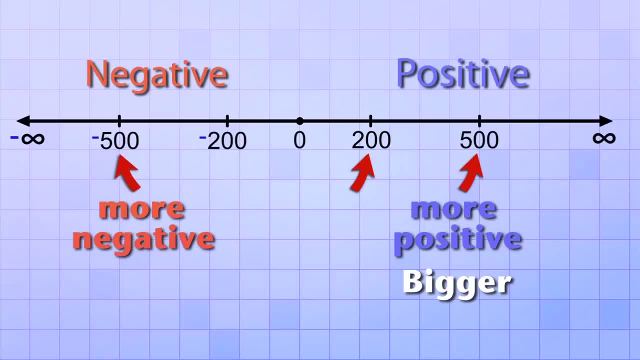 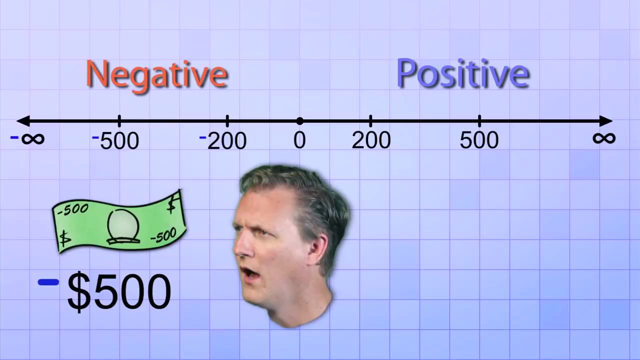 But on the negative side, negative 500 is more negative than negative 200, so it's smaller. Keep that in mind if anyone ever offers to give you negative $500.. The 500 part sounds pretty good, but the negative part… not so much. 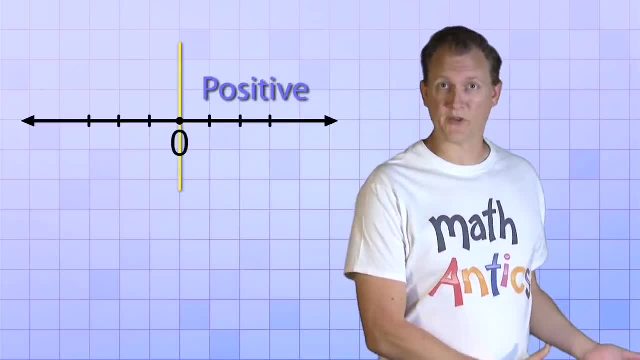 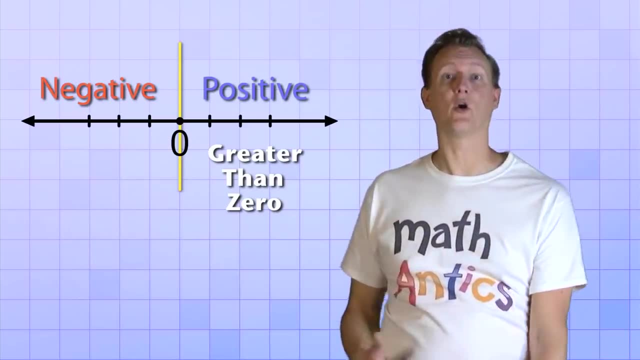 Alright, so the positive integers are on the right side of 0 on the number line, which means they're all greater than 0.. And the negative integers are all on the left side of 0 on the number line, which means they're all less than 0.. 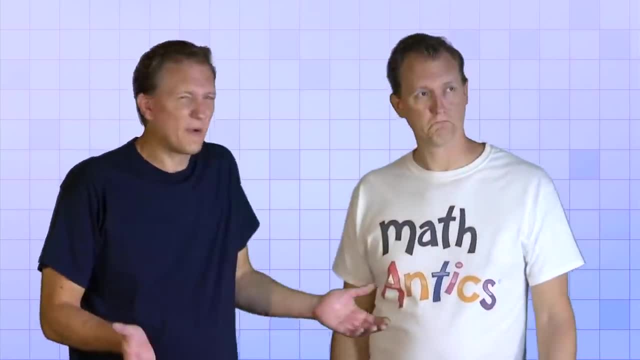 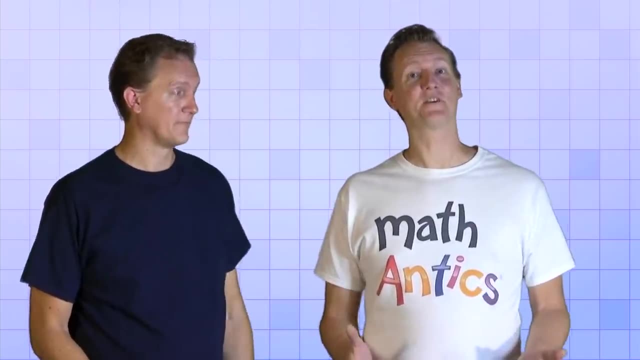 What Hold on a second Less than 0?? How can any number be less than 0?? I mean, doesn't 0 mean nothing? Ugh, that's a good question. At first it can be hard to see how there could be numbers that are less than 0.. 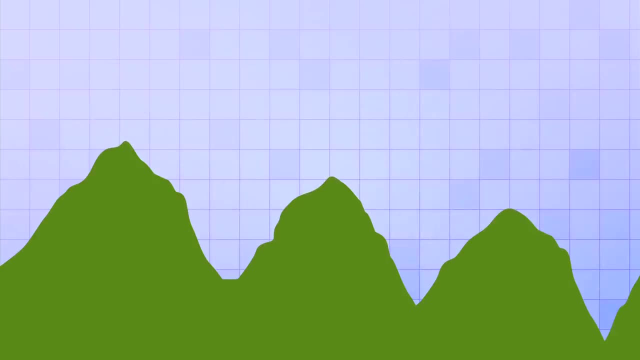 But here's an example that will help you understand. Let's say we want to use integers to measure how many meters above sea level small islands are. This island is 10 meters above sea level. This island is only 5 meters above sea level. 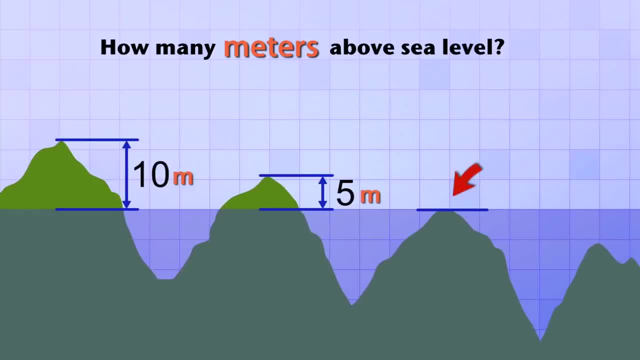 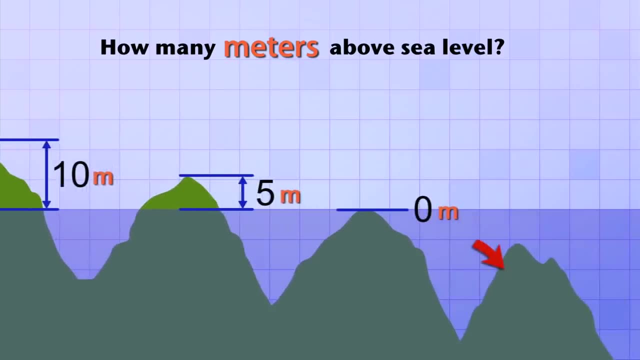 And this island here happens to be exactly the same height as sea level, So we can use the integer 0 to show how its height compares to sea level. But what about this island? It's not even above sea level at all. It's 5 meters below the surface. 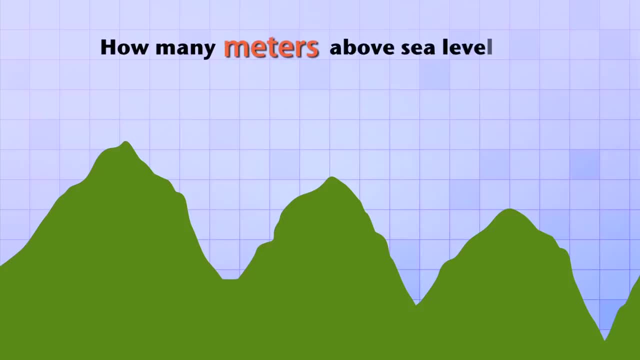 Let's say we want to use integers to measure how many meters above sea level small islands are. This island is 10 meters above sea level. This island is only 5 meters above sea level And this island here happens to be exactly the same height as sea level. 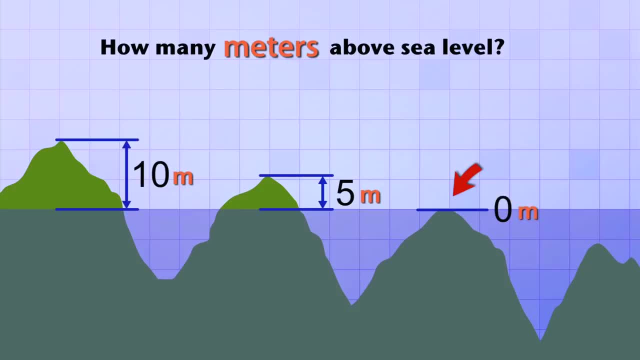 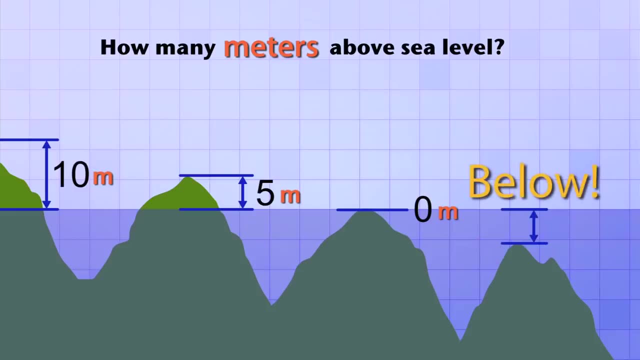 So we can use the integer 0 to show how its height compares to sea level. But what about this island? It's not even above sea level at all. It's 5 meters below the surface. But our measurement is supposed to tell us how many meters above sea level it is. 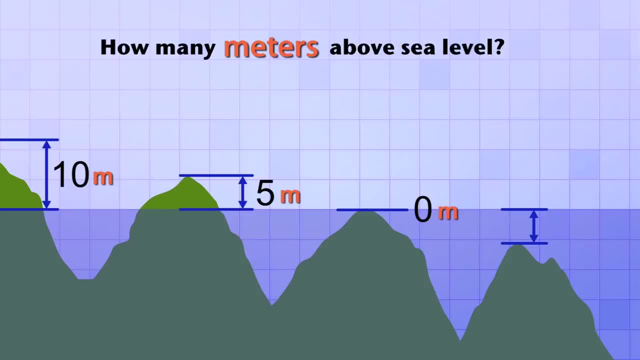 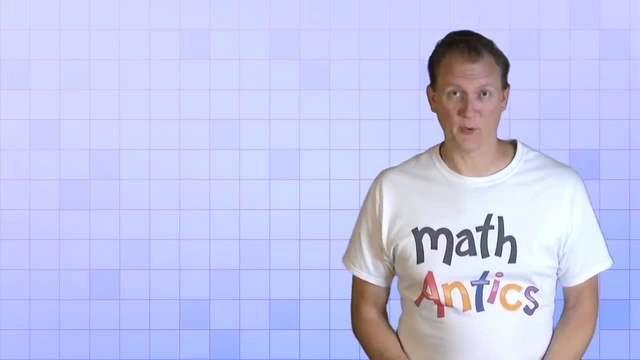 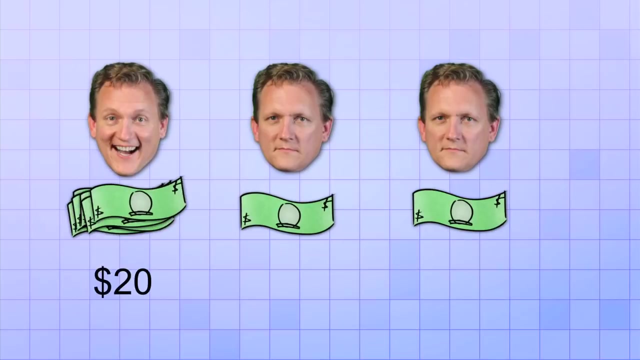 Fortunately, with negative numbers, that's no problem. We can just say that its height compared to sea level is negative 5 meters. Or what about an example with money? Suppose there's three brothers who each have a different amount of money. The first brother has $20. 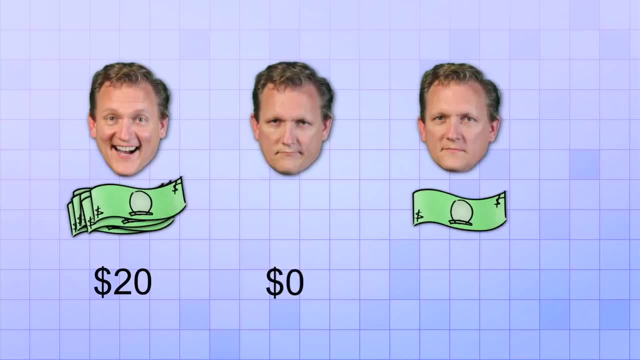 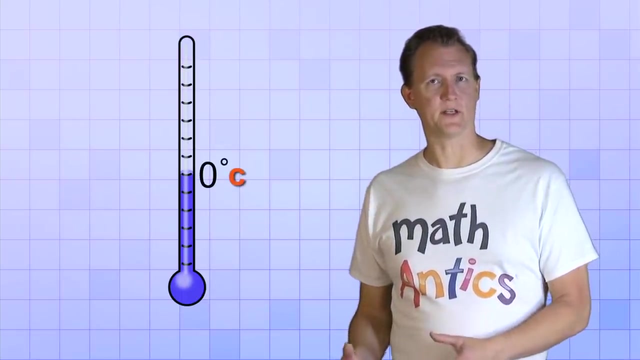 The next brother has $0.. And the last brother actually owes his dad $20.. What number do we use to represent how much money he has? Yep, negative $20.. And temperature is another great example. We use zero degrees Celsius to describe the temperature for water to freeze. 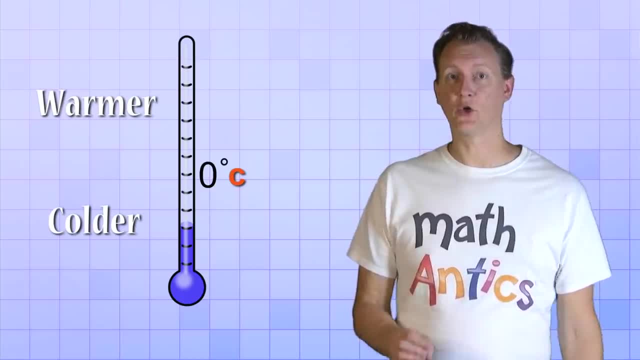 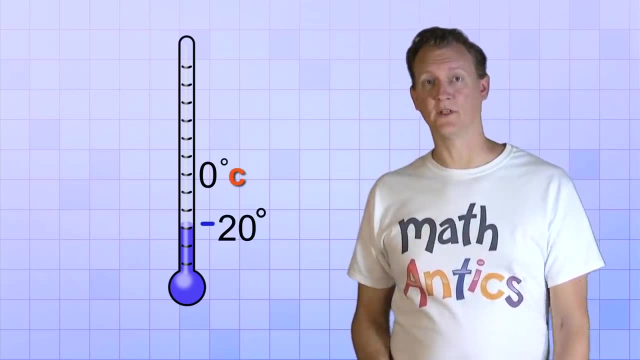 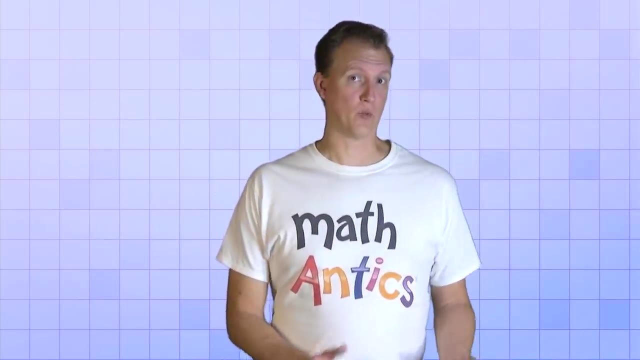 but it can be warmer or colder than that. The temperature could be negative, like negative 20 degrees. So negative numbers are very useful in the real world to help describe things that can be above or below zero. Okay, now that you know how negative numbers work, 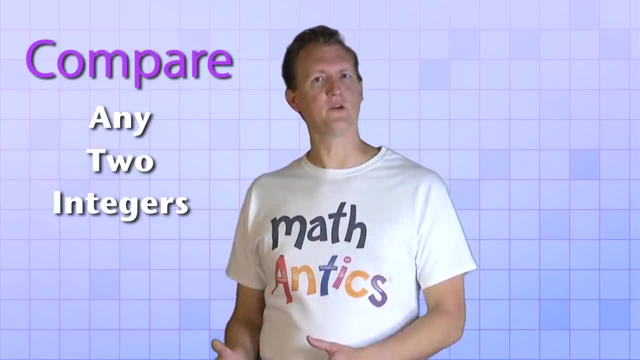 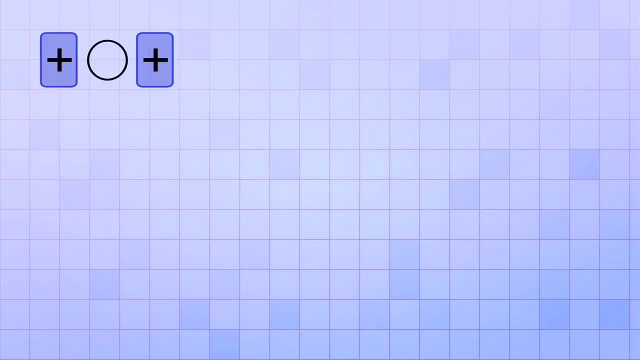 let's see how we can compare any two integers If we don't include zero for a moment. basically, there's just three situations. You'll either need to compare two positive integers or two negative integers, or one positive and one negative integer. 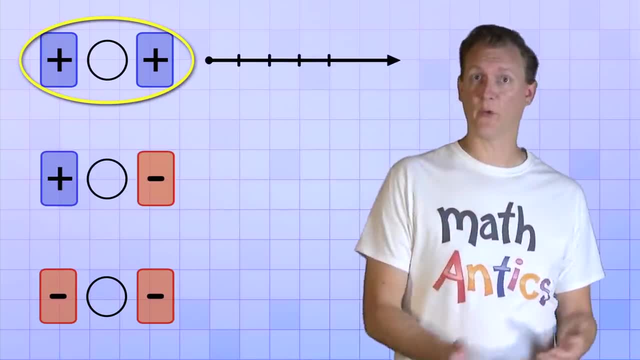 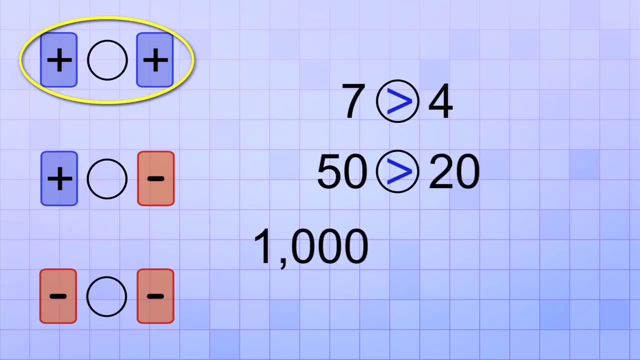 And you already know how to compare two positive integers. The further right on the number line you go, the bigger the numbers get: 7 is greater than 4,, 50 is greater than 20, and 1000 is greater than 100. 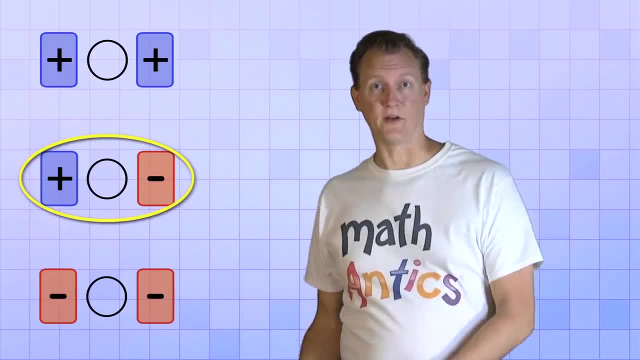 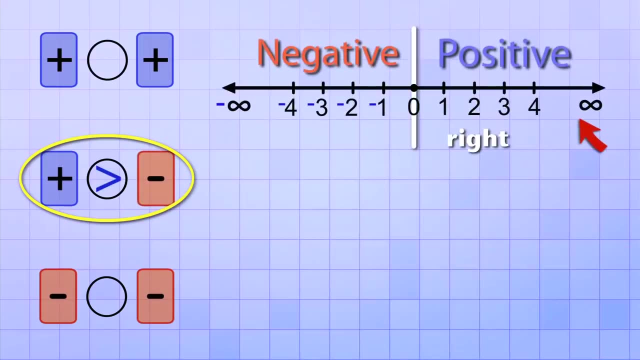 It's also really easy to compare a positive integer and a negative integer, because a positive number is always bigger than a negative number. All of the positive numbers are on the right side of the number line and all of the negative numbers are on the left. 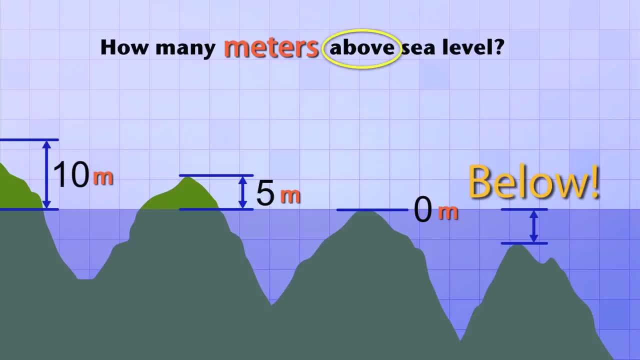 But our measurement is supposed to tell us how many meters above sea level it is, Fortunately with negative numbers, that's no problem. We can just say that its height compared to sea level is negative 5 meters. Or what about an example with money? 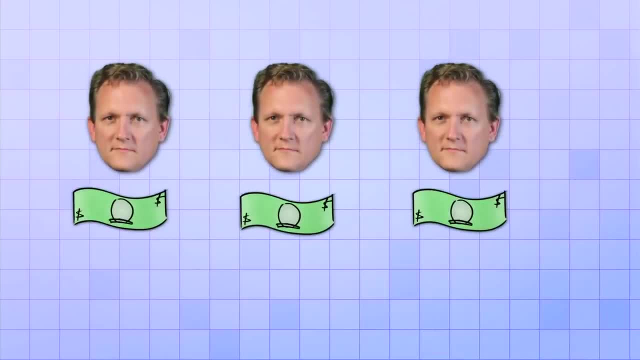 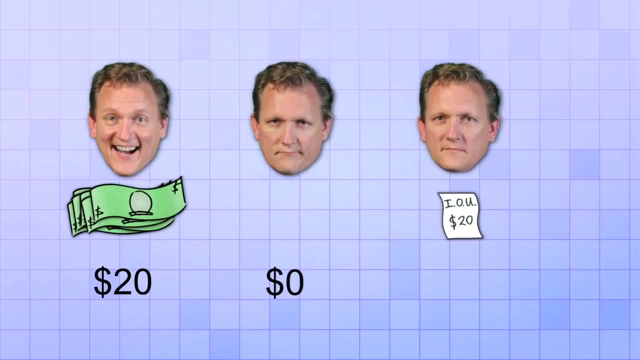 Suppose there's three brothers who each have a different amount of money. The first brother has $20,, the next brother has $0, and the last brother actually owes his dad $20.. What number do we use to represent how much money he has? 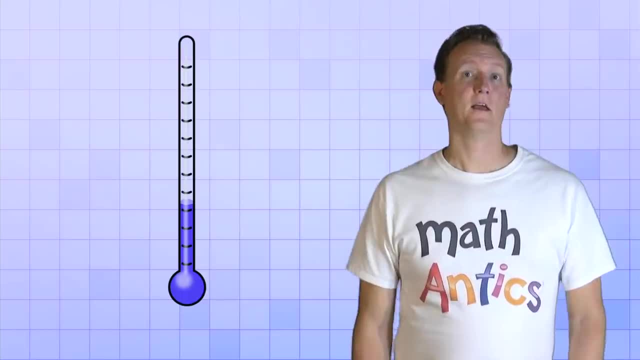 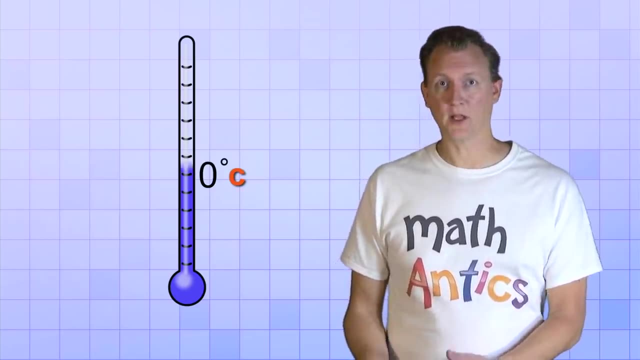 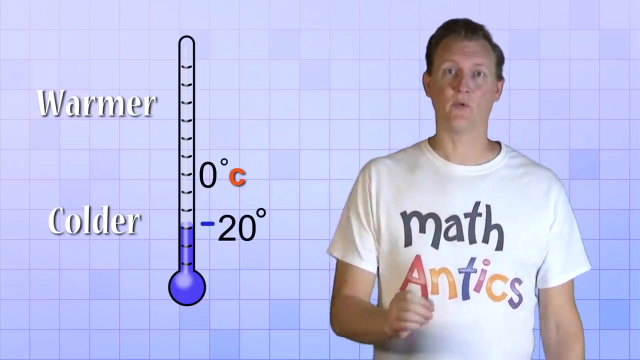 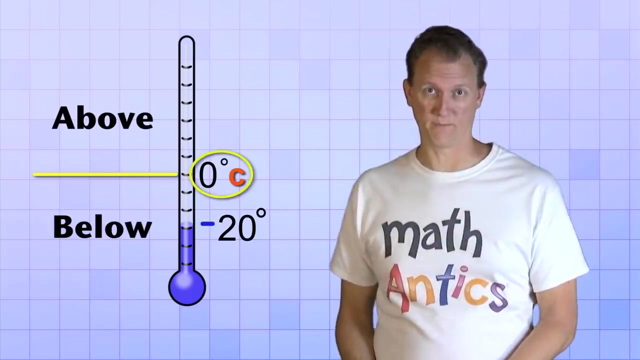 Yep: negative $20.. And temperature's another great example. We use 0 degrees Celsius to describe the temperature for water to freeze, but it can be warmer or colder than that. The temperature could be negative, like negative 20 degrees. So negative numbers are very useful in the real world to help describe things that can be above or below 0. 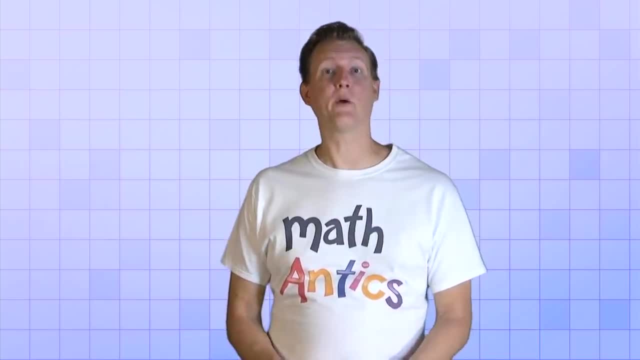 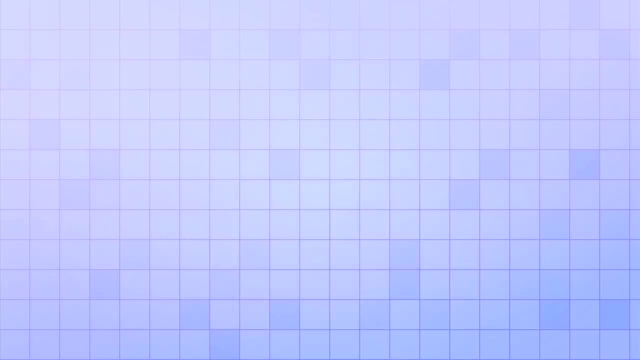 Okay, now that you know how negative numbers work, let's see how we can compare any two integers If we don't include 0 for a moment. basically, there's just three situations. You'll either need to compare two positive integers or two negative integers, or one positive and one negative integer. 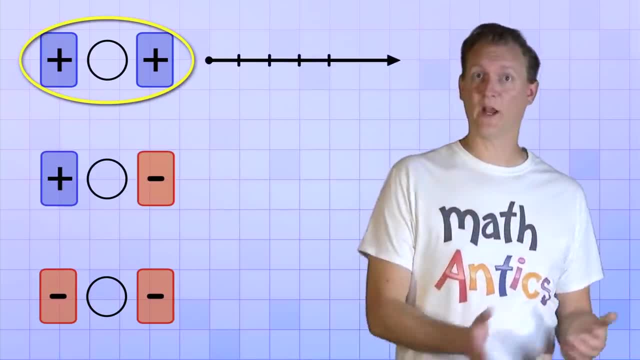 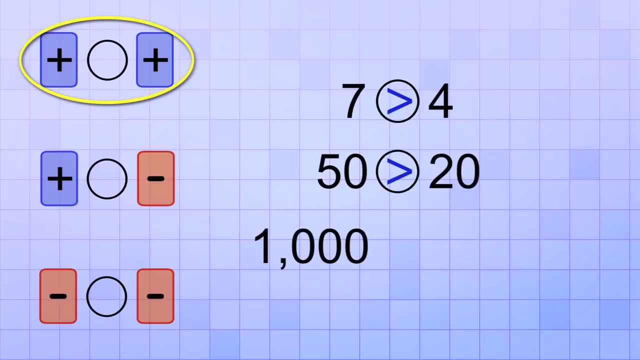 And you already know how to compare two positive integers. The further right on the number line you go, the bigger the numbers get: 7 is greater than 4,, 50 is greater than 20, and 1000 is greater than 100. 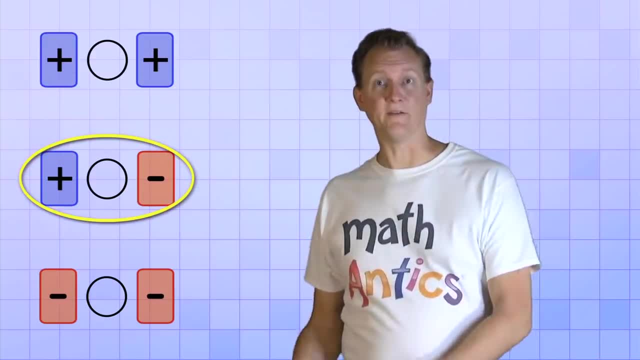 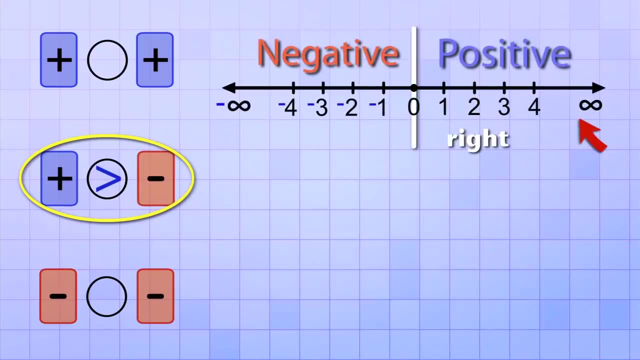 It's also really easy to compare a positive integer and a negative integer, because a positive number is always bigger than a negative number. All of the positive numbers are on the right side of the number line and all of the negative numbers are on the left. 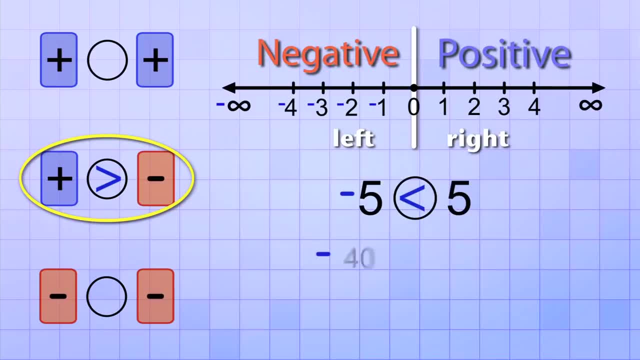 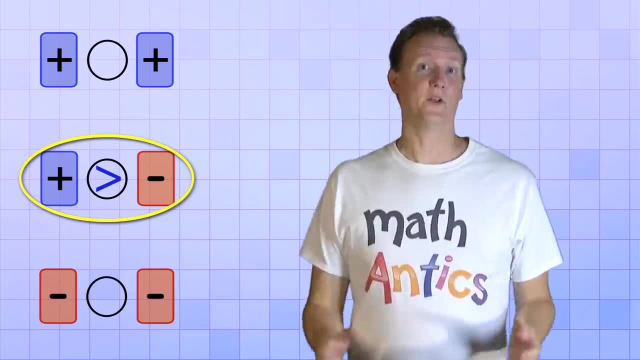 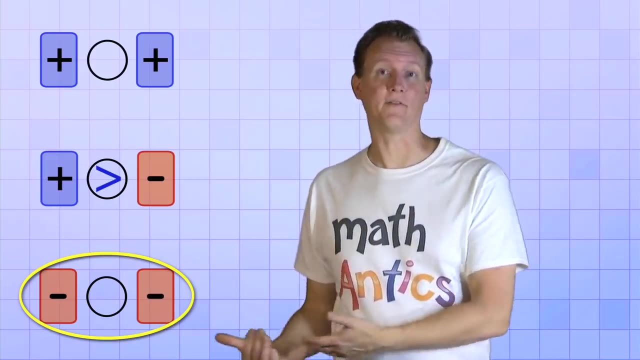 So negative 5 is less than 5, and negative 40 is less than 3, and negative 100 is less than 1.. The only tricky situation is when you have to compare two negative integers. Then you have to think about which one is further to the left on the number line. 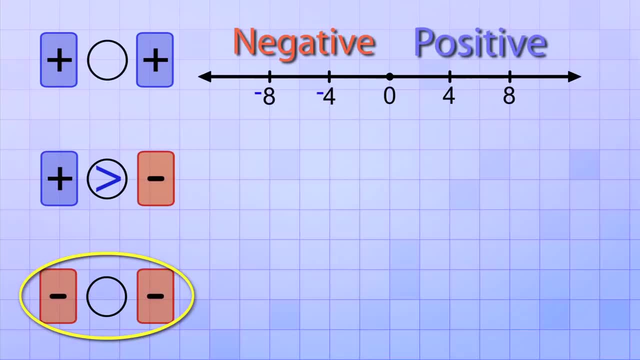 Again, a great way to do that is to identify the number that would normally be more positive on the positive side of the number line and realize that it's more negative on the negative side. Negative 8 is more negative than negative 4, so it's smaller.